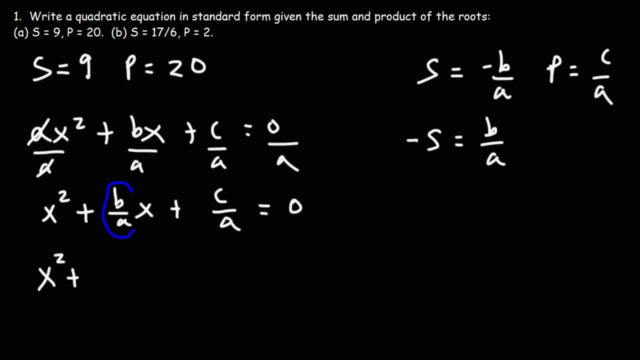 So I'm going to replace positive b over a with negative s And c over a. I can replace that with p, And this is the sum, And this is going to equal 0.. So if you're given the sum and the product of the roots, you could simply use this formula to write the quadratic equation. 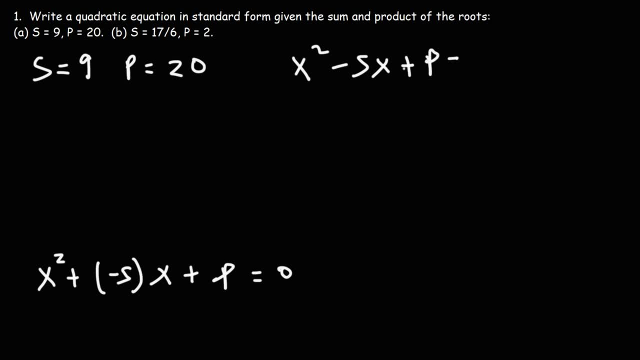 x squared minus sx plus p is equal to 0, where s is the sum and p is the product. So replace the sum and the product. So replace the sum and the product. So if we replace s with 9, we have negative sx, or 9x plus p, p is 20, and this is equal to 0.. 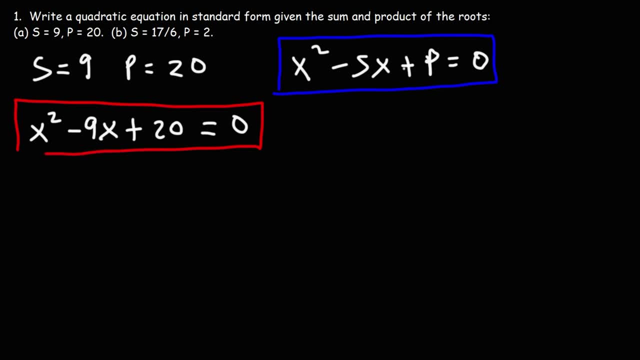 So this right here is our answer, But let's confirm that we have the right answer. So what I'm going to do is I'm going to factor this quadratic equation and then I'm going to solve it And then, using the roots, I'm going to confirm that the roots are correct. 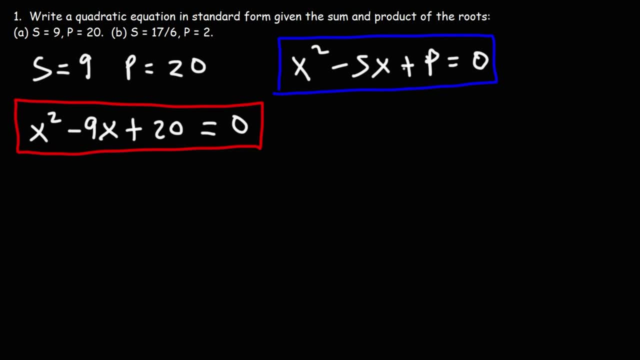 So in order to factor this trinomial, we need to find two numbers that multiply to 20, but add to the middle coefficient 9.. So if we divide 20 by 1,, we get 20.. If we divide it by 2,, we get 10.. 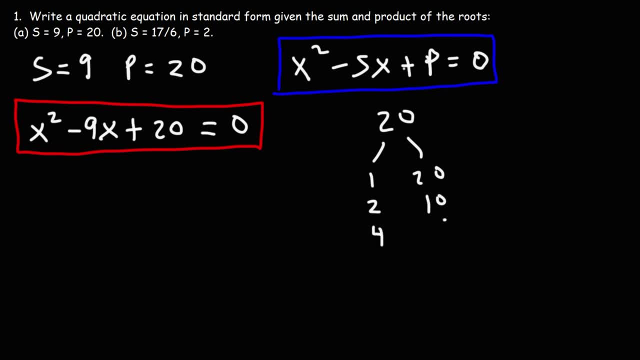 20 divided by 3 doesn't give us a whole number, but if we divide it by 4, we get 5.. Now 4 plus 5 adds up to 9.. So if we divide 20 by negative 4, we get negative 5.. 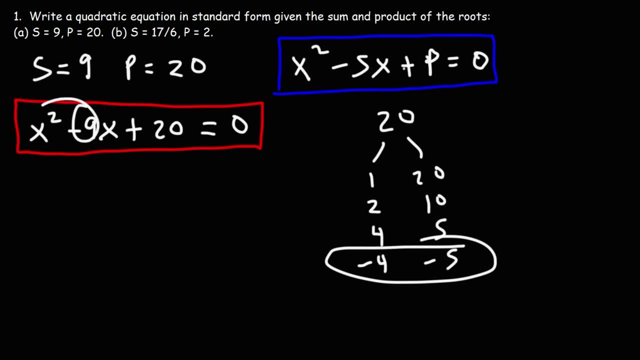 But negative 4 and negative 5 adds up to negative 9.. So those are going to be used for our factors. So what I'm going to do is I'm going to replace negative 9x with negative 4x and negative 5x. 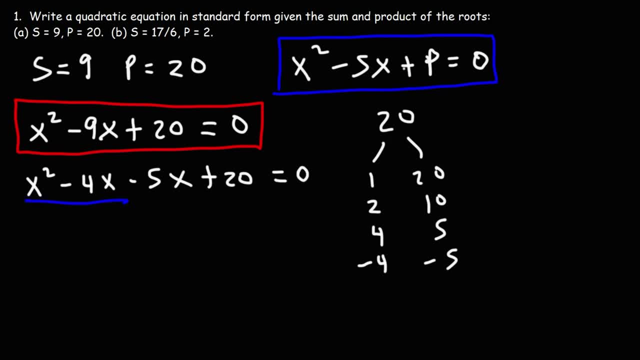 And then I'm going to factor by grouping. So, in the first two terms, I'm going to take out an x: x squared divided by x is x Negative 4x divided by x is negative 4.. And then, in the last two terms, I'm going to take out the GCF, the greatest common factor. 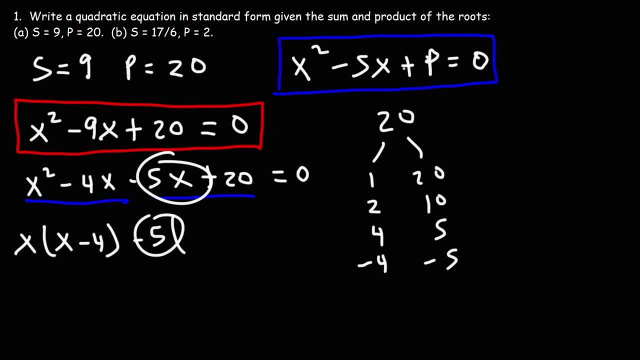 And that's going to be negative 5.. Negative 5x divided by negative 5 is x 20. divided by negative 5 is negative 4.. Next, I'm going to factor out x minus 4, since that's a common factor. 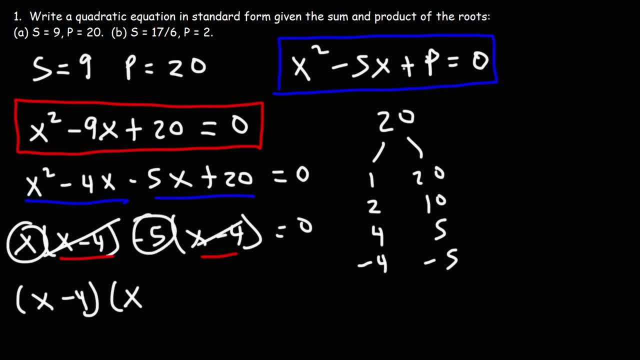 Once I do that, I'll be left with x minus 5.. So if the leading coefficient is 1,, once you get these two numbers, you can simply write it like this in factored form: Now, using the zero product property, we're going to set each factor equal to 0.. 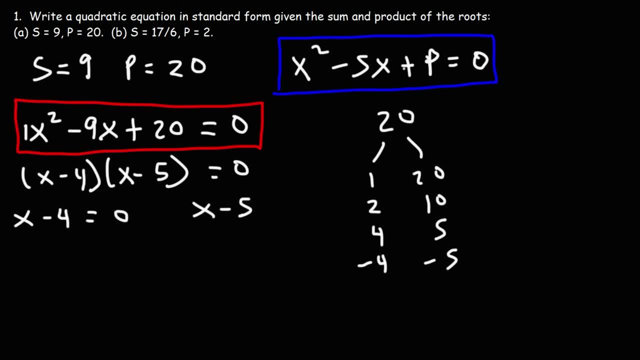 And we're going to solve for x. Add in 4 to both sides, We get that the first root, which we'll call x sub 1, is 4.. Add in 5 to both sides in the other equation, We'll get that the second root, which we'll call x sub 2, is 4.. 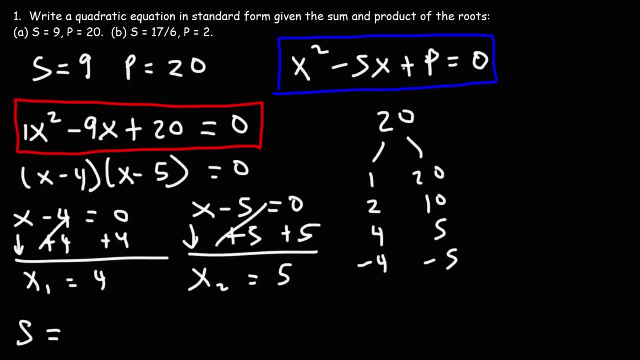 x sub 2 is 5.. Now the sum of these two roots- 4 plus 5, gives us 9,, as we can see here, And the product of these two roots 4 times 5, will give us 20.. 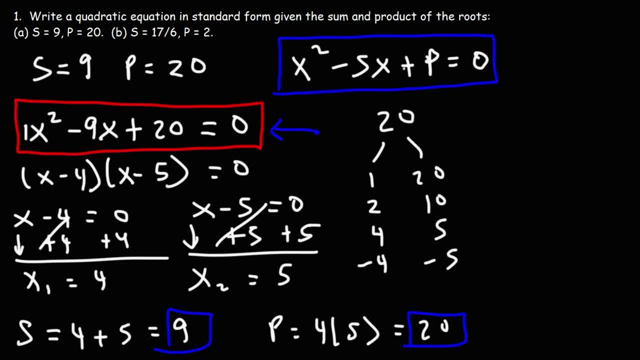 So that's how we can confirm if we have the right quadratic equation. But the answer that we're looking for in this problem for part A is what we have highlighted here: x squared minus 9x plus 20 is equal to 0.. 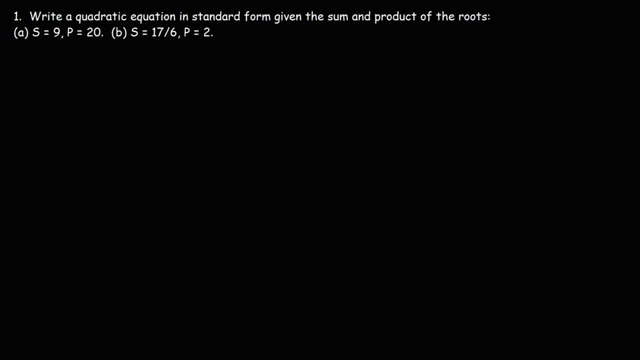 Now let's try a harder example. Let's move on to part B. So using the formula x squared minus sx plus p is equal to 0.. We have that s the sum of the roots is 17 over 6.. 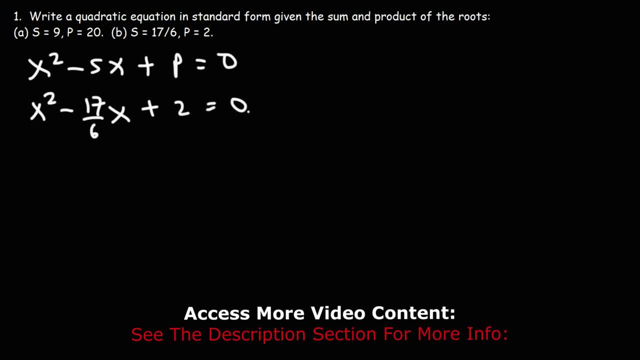 And the products. I mean the product is 2.. Now we can't leave our answer like this, because we want to get rid of this fraction, to put it in standard form. To do that, I'm going to multiply everything by 6.. 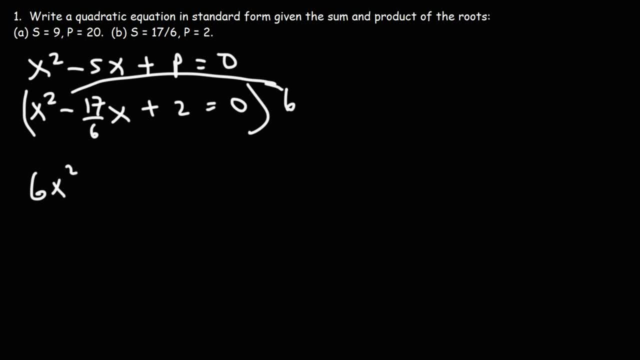 So we're going to have 6x squared Now, 6 times 17 over 6, the 6 will cancel, giving us just 17.. And then 6 times 2 is 12.. And 0 times 6 is still 0.. 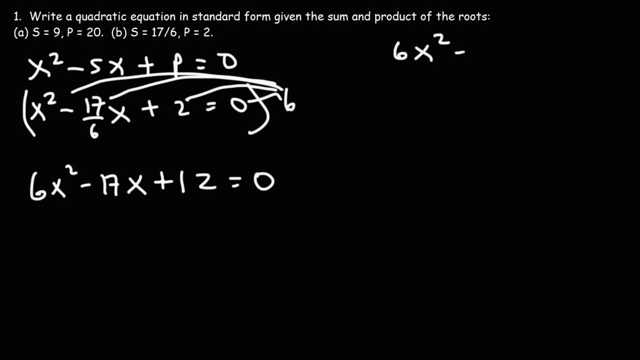 So this is going to be our answer: 6x squared minus 17x plus 12 is equal to 0.. That's the answer for part B. All we need to do now is confirm that this answer is correct. In order to do that, I'm going to factor it using the AC method. 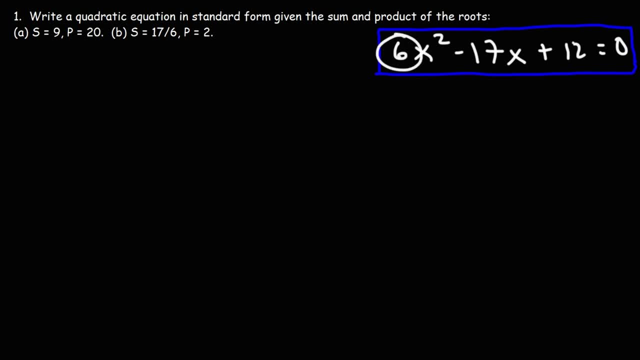 With the AC method we're going to multiply the A coefficient by the constant See, So that's 6 times 12, which is 72. And we need to find two numbers that multiply to 72, but add to the middle coefficient negative 17.. 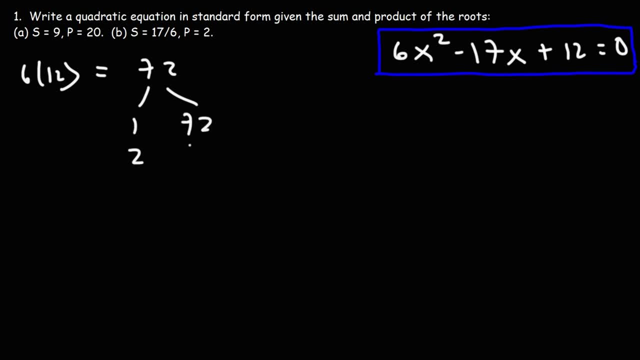 So if I divide 72 by 1,, I get 72.. If I divide it by 2, I get 36.. If I divide it by 3,? if you're not sure what it's going to be, here's what you can do. 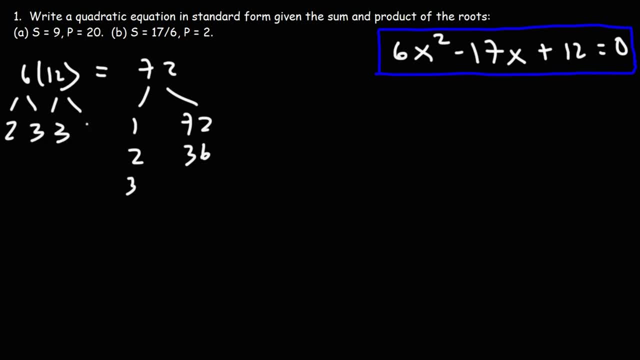 You can break up 6 into 2 and 3, and 12 into 3 and 4.. So if I take out 1,, I get 3.. What I have left over is 4 times 3,, which is 12,, times 2,, which is 24.. 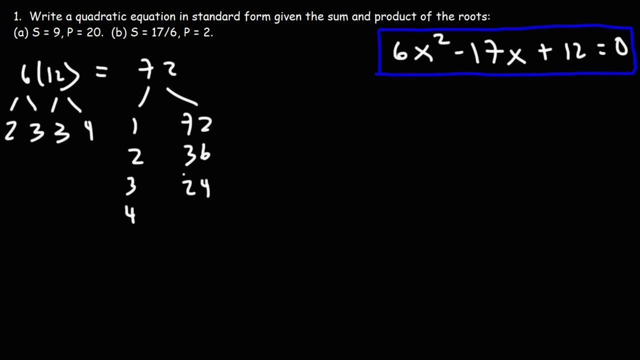 So 72 divided by 3 is 24.. If we divide it by 4, we're left with 2 times 3 times 3, which is 3 times 3 is 9, times 2 is 18.. 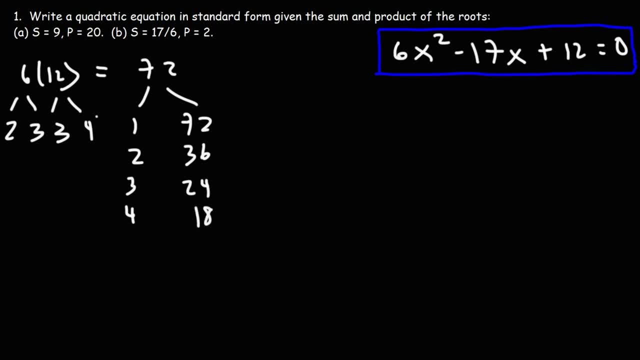 So 72 divided by 4 is 18.. Now there's no 5 in here, so 72 won't be divisible by 5. It is divisible by 6.. We can see: 6 times 12 is 72.. 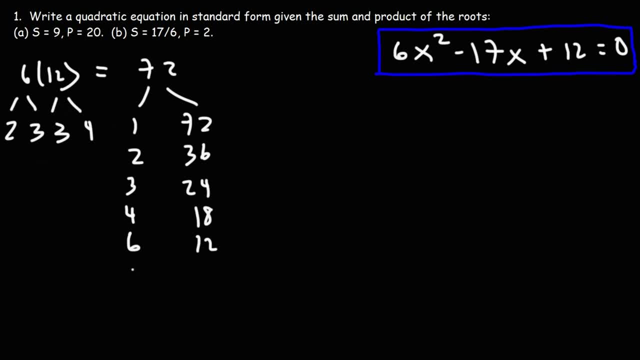 We can't get it right. We can't get a 7 here, so that's out. We can get an 8.. 2 times 4 is 8, and 3 times 3 is 9,, so 9 is left over. 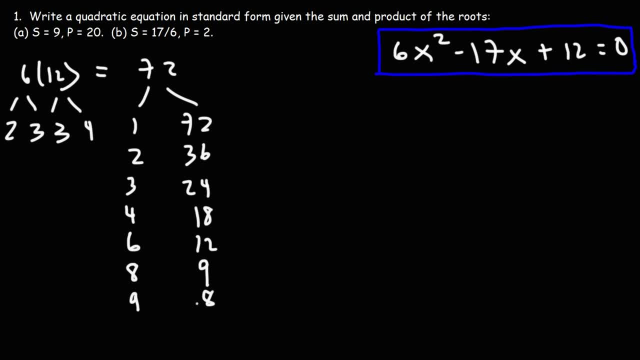 Once it begins to reverse, you pretty much have everything that you need. Now it needs to add up to negative 17.. 8 plus 9 is positive 17.. But negative 8 and negative 9 adds up to negative 17.. 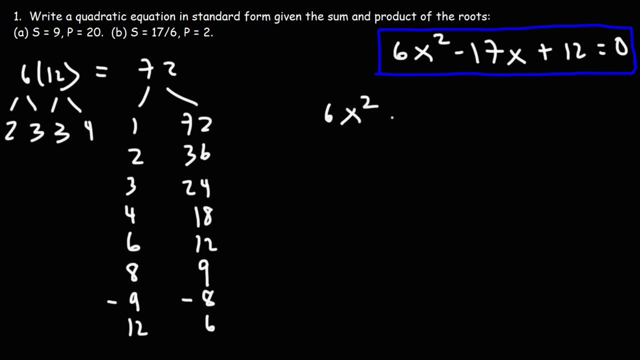 So to factor it, we're going to replace negative 17x with negative 9x and negative 8x, And then let's factor by grouping. In the first two terms, the GCF is going to be 3x. 6x squared divided by 3x is 2x. 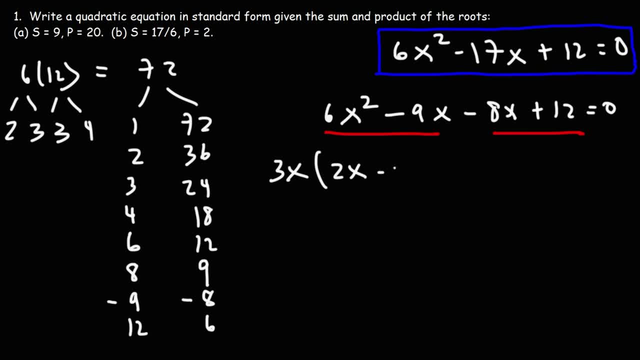 Negative 9x divided by 3x, That's going to be Negative 3.. In the last two terms I'm going to take out negative 4.. Negative 8x divided by negative 4 is 2x. Positive 12 divided by negative 4 is negative 3.. 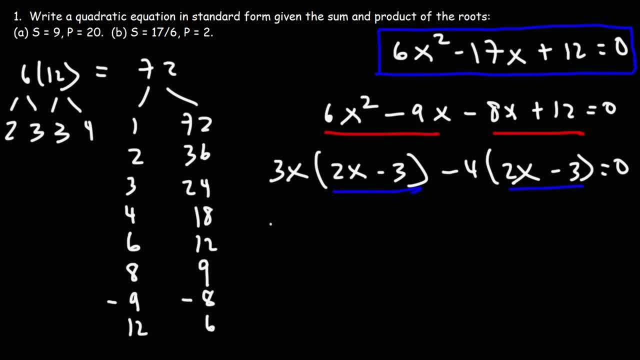 So now we're going to factor out the GCF again, which, now that we have the common factor 2x minus 3, we're going to be left with 3x once we take it out of the first term. When we take out 2x minus 3 from the second term, we're left with negative 4.. 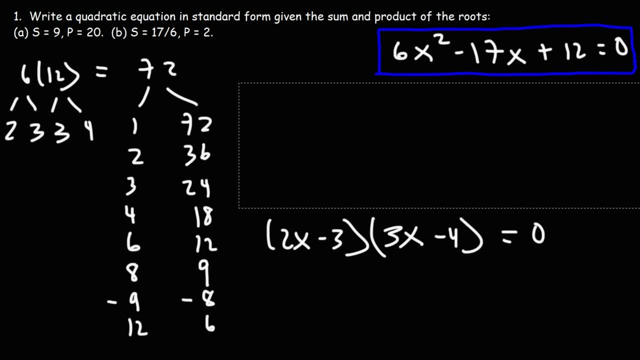 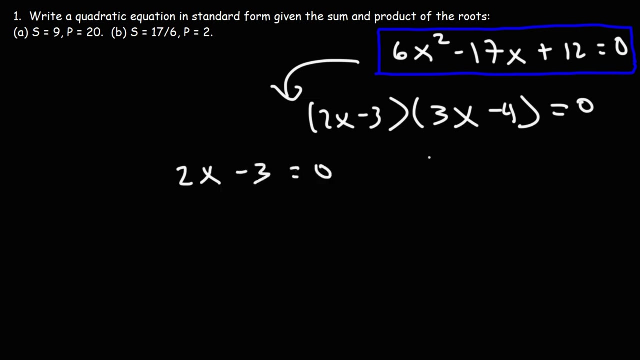 Negative 3.. So 6x squared minus 17x plus 12 can be factored into this expression. So now, using the zero product property, I'm going to set each factor equal to 0.. and then solve for x. so first i'm going to add 3 to both sides, i'm going to get 2x is equal to 3. 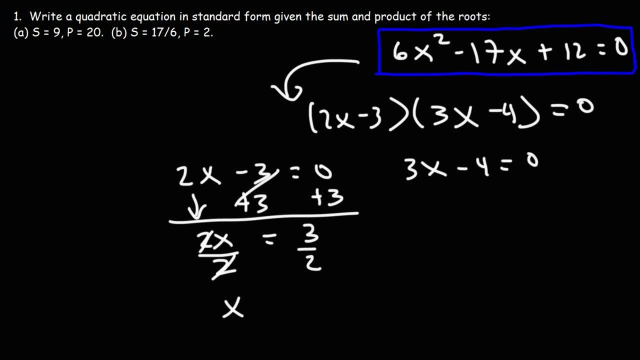 and then i'm going to divide both sides by 2. so the first root is that x is 3 over 2. for the next one, i'm going to add 4 to both sides, bring down to 3x, so we have 3x is equal to 4, and then i'm 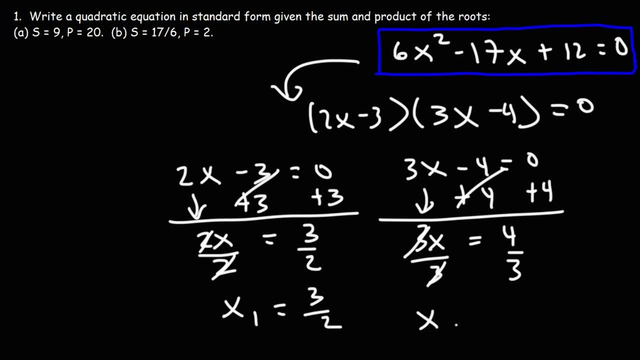 going to divide both sides by 3. so the second root is that x is 4 over 3. so now let's get the sum and product. so the sum is going to be the sum of these two numbers. it's 3 over 2 plus 4 over 3. to add these fractions we need to get common denominators. 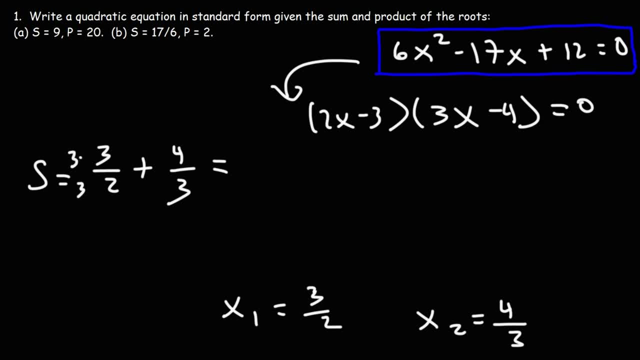 so let's get a common denominator of 6, which means i need to multiply this by 3 over 3 and this one by 2 over 2, So we have 9 over 6 plus 8 over 6,. 9 plus 8 is 17,, and we can see that this value is confirmed. 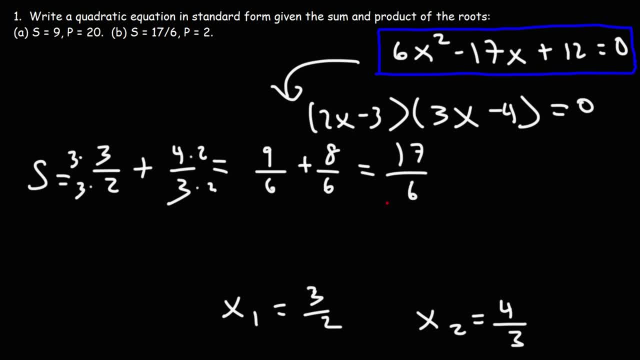 This should be 17 over 6, which is what we have here. Now let's calculate the product. It's 3 over 2 times 4 over 3.. Multiplying across, we could cancel the 3's, and so we're left with 4 over 2, 4 divided by 2 is 2..